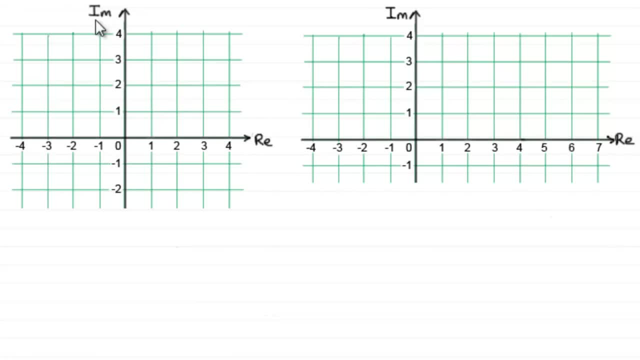 But I'm going to keep mine as RE and IM. So if we had a complex number, let's just say we had the complex number Z1, equaling 3 plus 2I. We represent this on an argon diagram by going 3 units in the positive real sense. 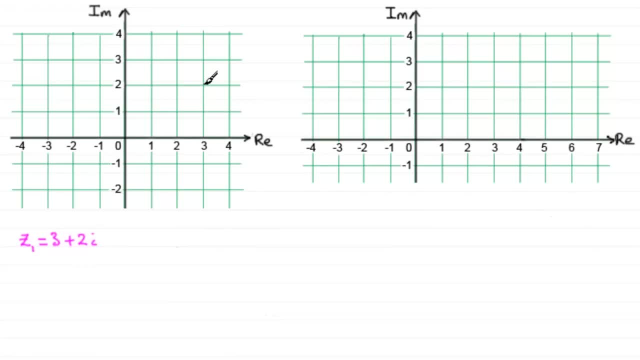 and 2 units in the positive imaginary sense And it's represented by a negative real sense And it's represented by a positive imaginary sense And it's represented by a negative real sense. And it's represented by a negative imaginary sense And it's represented by a negative real sense. 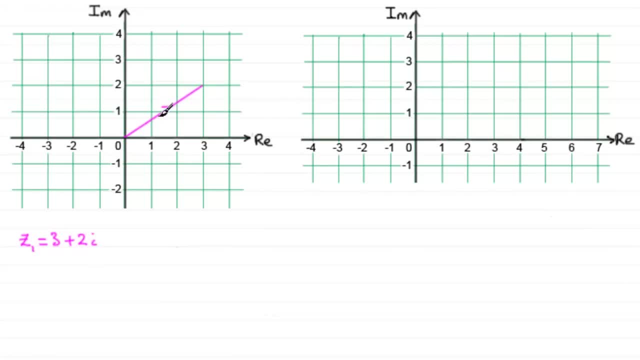 And it's represented by a line, A line with an arrow, So it looks like a vector. It has length and direction. So this would be how we represent Z1 then on an argon diagram. Suppose I did the complex conjugate of Z1, often written Z1 with a little star. 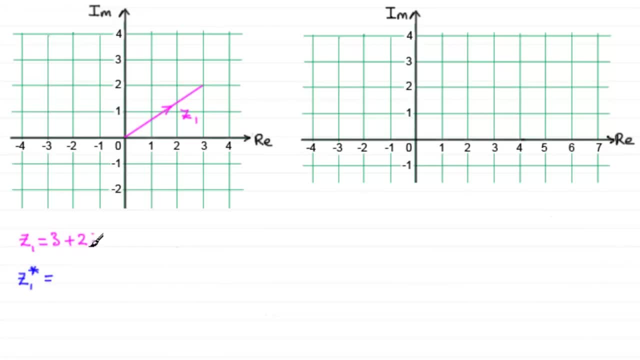 Remember that when you have a complex conjugate of a complex number, all you do is you switch the sign of the imaginary part. so we end up with 3 minus 2i, And if we were to draw this on the Argon diagram, it would look something like this: 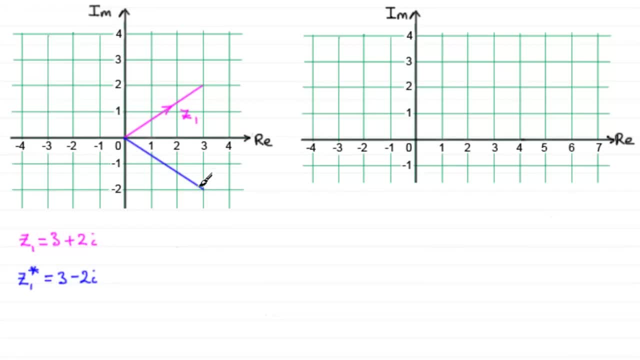 Three units across, two units down. Don't forget the arrow. and this would be the complex conjugate of Z1.. And do you notice how it's related to Z1? It's a reflection in the real axis. Now, if we had another complex number, let's say Z2.. 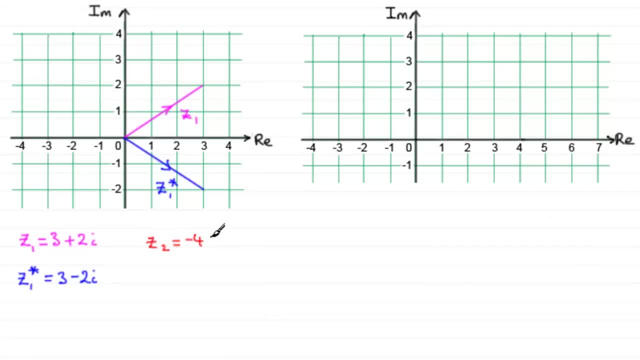 Z2 was equal to minus 4 plus i And we were to draw this on the Argon diagram, Then we'd go minus 4 and plus one unit up there. So going from there to there would be our complex number Z2.. 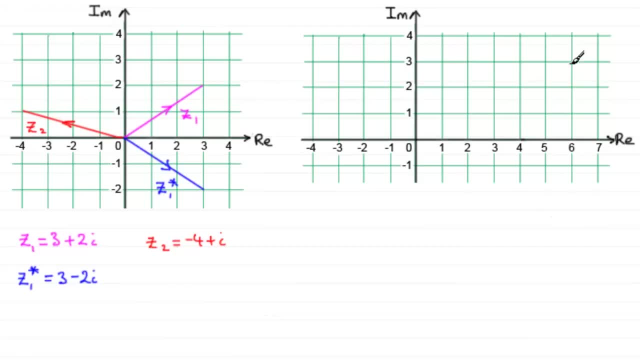 Now if we were to add Z1 and Z2 together, let's just do that Z1 plus Z2.. What do we get? Well, 3 minus 4 is minus 1, and 2i plus i is 3i. 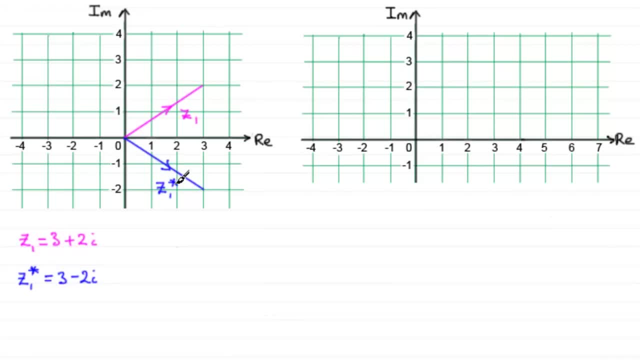 conjugate of Z1.. And do you notice how it's related to Z1?? It's a reflection in the real axis. Now, if we had another complex number, let's say Z2.. Z2 was equal to minus 4 plus i, And we were to draw this on the argon. 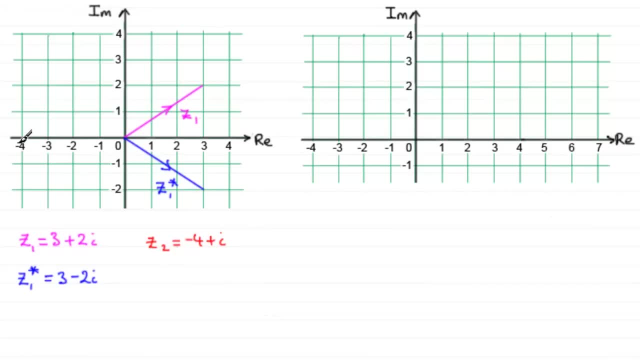 diagram. Then we'd go minus 4 and plus 1 unit up there. So going from there to there would be our complex, So we'd get our complex number Z2.. Now, if we were to add Z1 and Z2 together, 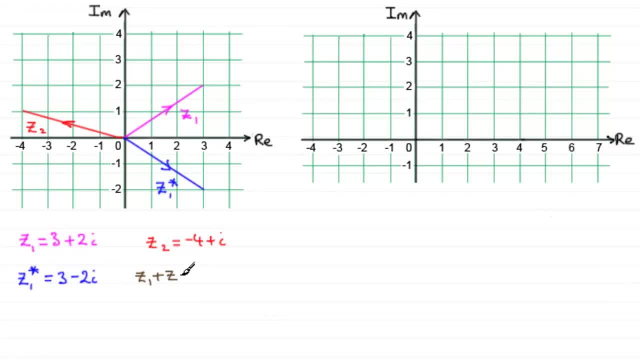 Let's just do that: Z1 plus Z2.. What do we get? Well, 3 minus 4 is minus 1.. And 2i plus i is 3i. And if we were to represent this on the argon diagram, 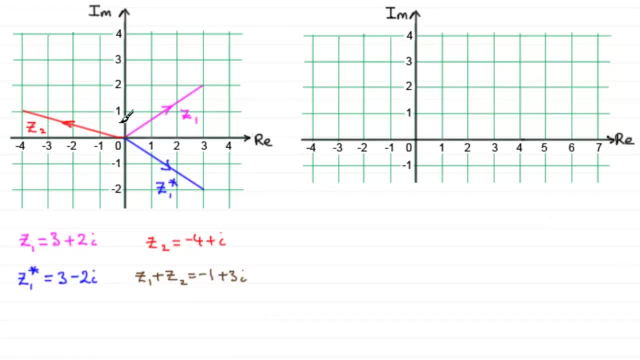 it would be something like this, like this: go from the origin up to there. okay, so that would be z1 plus z2. now it's very interesting to relate this to vectors. if I was to say, call z1 OA and z2 OB, then if I was to do o2a plus o2b- let's just put it down here. 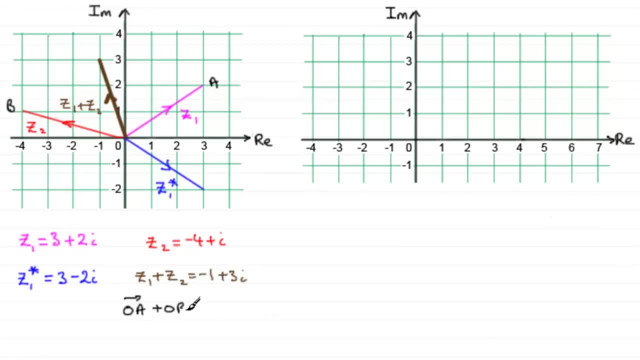 o2a plus o2b. remember, in vectors the plus means followed by. let's see what we get if I was to draw over z2 like. so just take a copy of it and now translate it across here. can you see that we're doing z1 followed by z2? what? 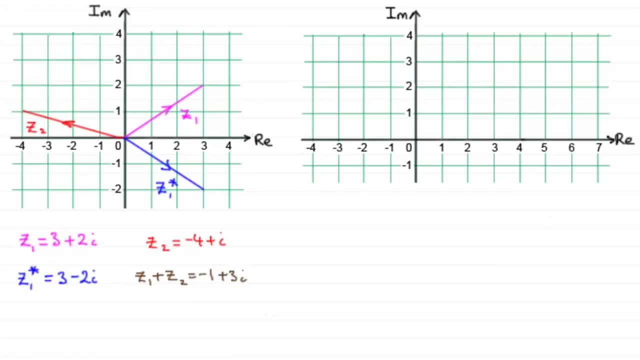 And if we were to represent this on the Argon diagram, it would be something like this: It's going from the origin up Two up there. OK, So that would be Z1 plus Z2.. Now it's very interesting to relate this to vectors. 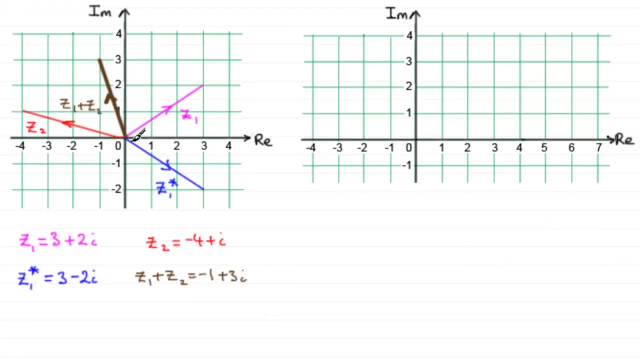 If I was to say: call Z1OA and Z2OB. if I was to say: call Z1OB and Z2OB. Then if I was to say: call Z2OA and Z2OB. Then if I was to say: call Z2OB and Z2OA. 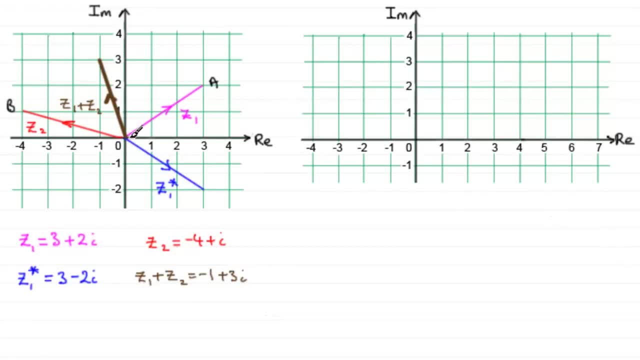 to do: o to a plus o to b. let's just put it down here: o to a plus o to b. remember, in vectors the plus means, followed by: let's see what we get if i was to draw over z2 like. so just take a copy of. 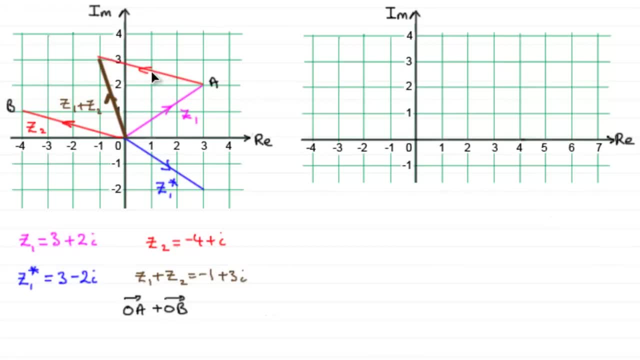 it and now translate it across here. can you see that we're doing z1 followed by z2. what we get is z1 plus z2. so in other words, if i called this point on the end here, c, z1 plus z2, o, c, then o to a plus o to b equals o to c. we didn't have to do this. 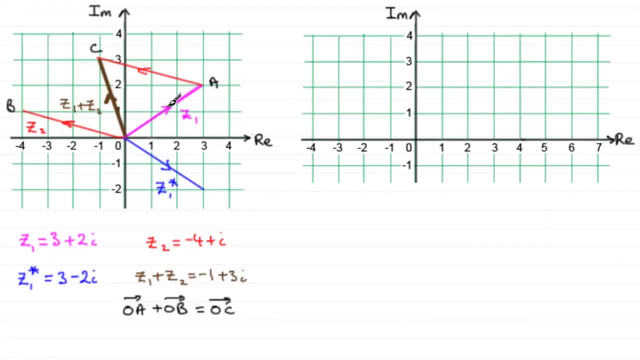 we could have even done z1, and we could have translated that across and done z2, followed by or plus z1. still the same result, this diagonal of the resulting parallelogram. so you can see, i hope, how complex numbers relate to vectors. now, having said that, suppose we look. at this vector and we can see that we have a vector that is equal to z1 and we can see that we have a vector that is equal to z1 and we can see that we have a vector that is equal to z1 and we can. 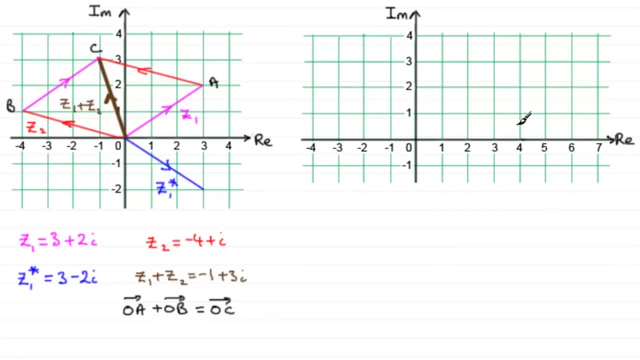 at this argon diagram and draw z1 and z2 back on again. now, if we do z1 minus z2, what do we get this time? well, three minus minus four is going to be seven, and two. i minus plus i is going to be plus. 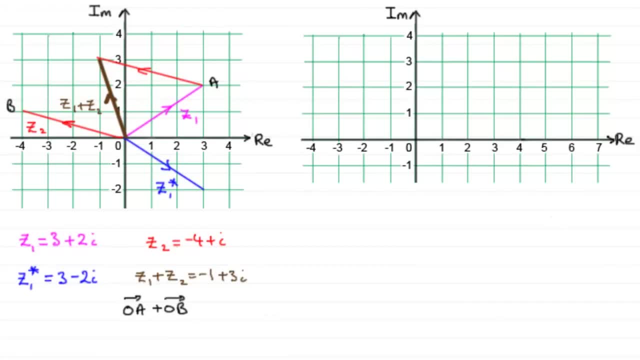 we get is z1 plus z2. so in other words, if I called this point on the end here- see z1 plus z2 OC- then o2a plus o2b equals o2c. we didn't have to do this, we could have even done z1 and we could have translated that across and done z2. 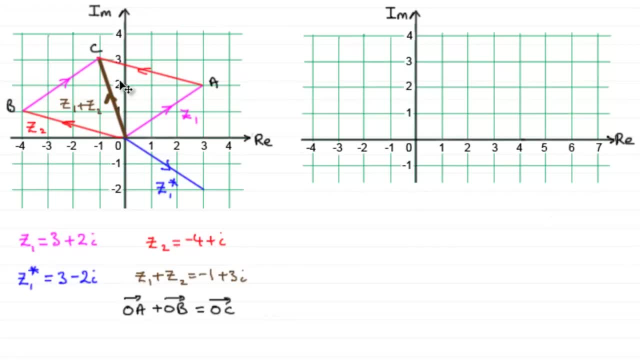 followed by or plus z1, still the same result, this diagonal of the resulting parallelogram. so you can see, I hope, how complex numbers relate to vectors. now, having said that, suppose we look at this argand diagram and draw z1 and z2 back on again. now, if we do z1 minus z2, what do we get? 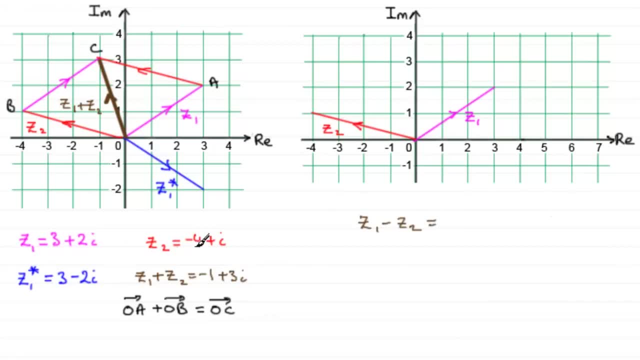 this time. well, 3 minus minus 4 is going to be 7, and 2i minus plus i is going to be plus i. and if we represent 7 plus i on the argand diagram, seven units here, one unit up, we've got this. so this is the complex number: z1 minus z2, but in the same way. 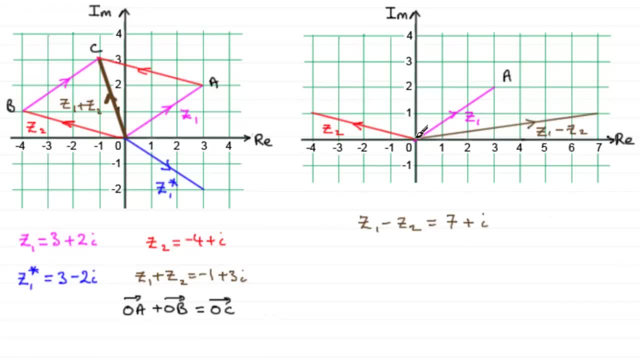 if z1 is o2a and z2 is o2b, if we were to take this vector, we can translate this over to here, and that fits in well with our vectors, because if I think what b to a is, b to a would be b to o followed. 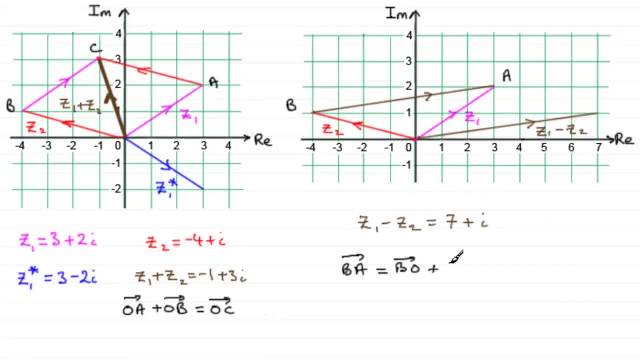 by o to a, and going from b to o is exactly the same as doing the reverse direction: minus o to b, followed by o to a, and we can swap this round as o to a, minus o to b, o to a being z1, then o to b being z2, z1 minus z2..